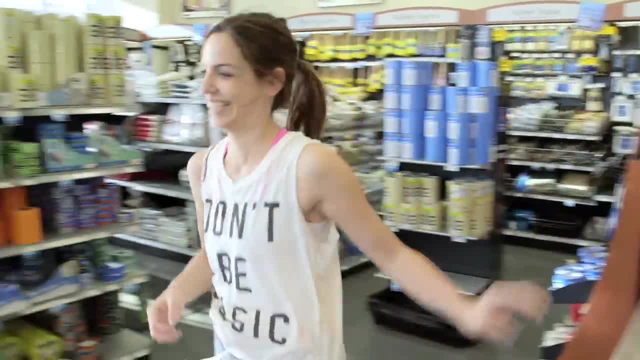 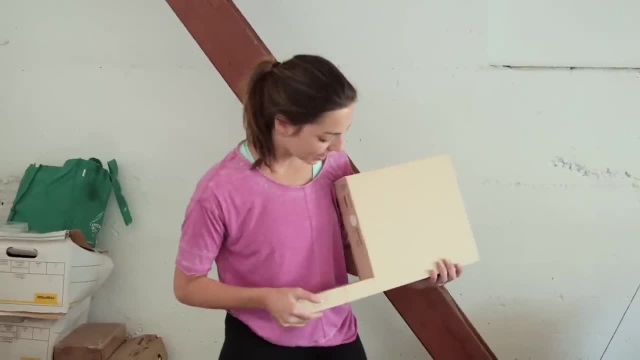 way, they're still on. Thank you cheers. Donation items. be realistic with the stuff that's just sitting down there- An un-put-together chair from Ikea. These needs to be donated to someone more handy. I had a lot of maybes from my closet purge. I had to have a little waiting period. 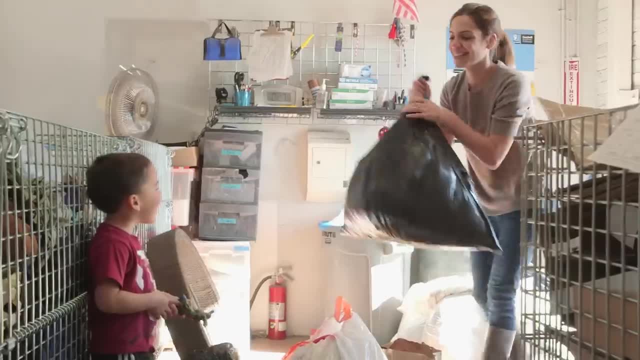 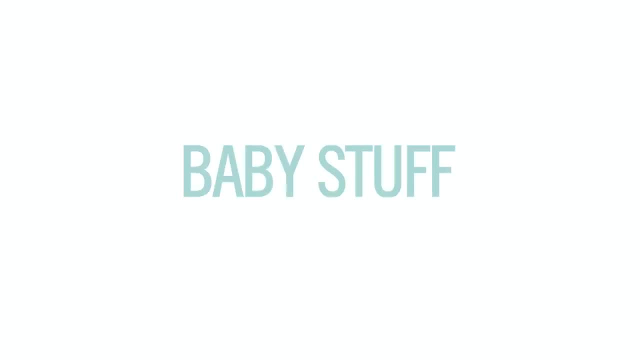 and no, I did not miss them. I finally took them to Goodwill. It's official And this is a great place to teach kids one way that they can help others. High five: Lots of baby stuff. Donate, need it anymore. I wanted to take some of my nicer strollers to the baby, to baby. 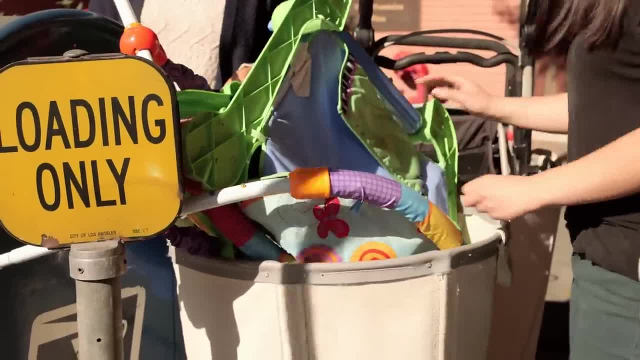 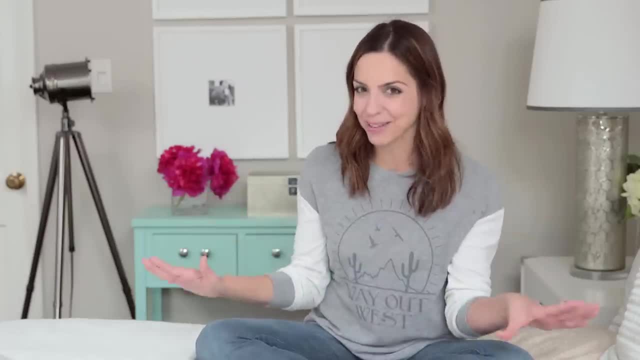 charity, because I knew it would find a fantastic home. Churches take these items or, of course, friends with younger kids. My tip here is to have them come pick it up on the day you're cleaning so that it actually happens. Recyclables, It's like. 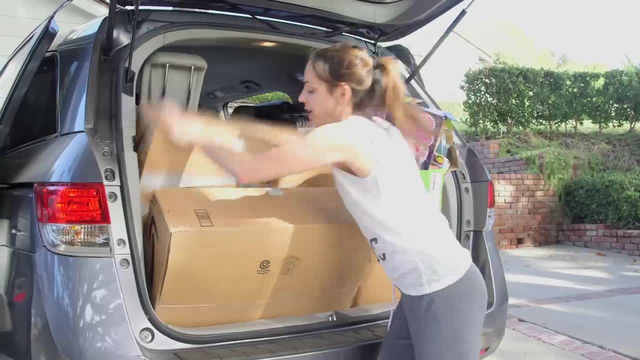 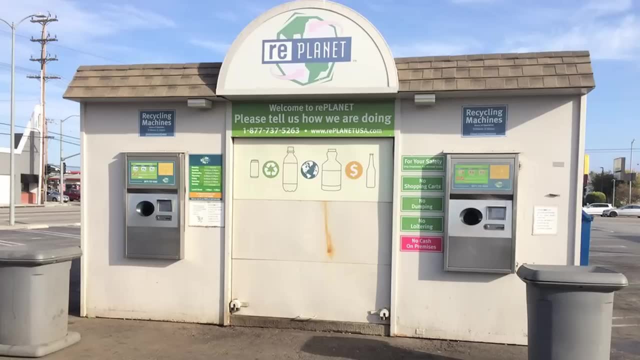 finding a gift, except when you have too many to fit into your bin. so I ended up piling them up in my trunk. googled recycling centers. thought I was going here, ended up finding myself in the hub of Santa Monica recycling and wow this. 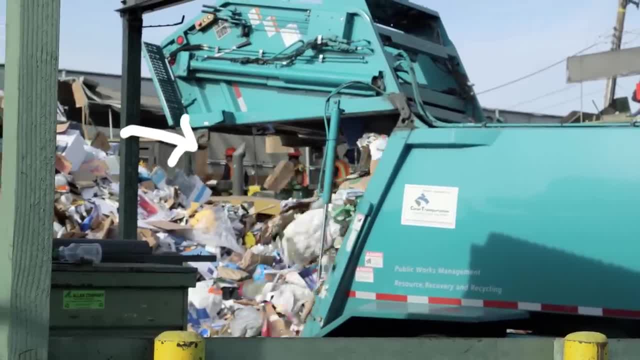 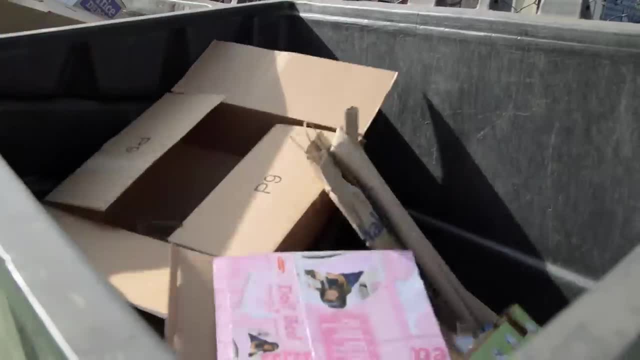 is definitely not how I imagined it. There were people sorting through all of the stuff and it gave me a new appreciation. I like feel bad ever putting anything anywhere. I was very glad to separate my items and put them in the label bins they had outside. Last but not least, husband stuff. This is the hardest. 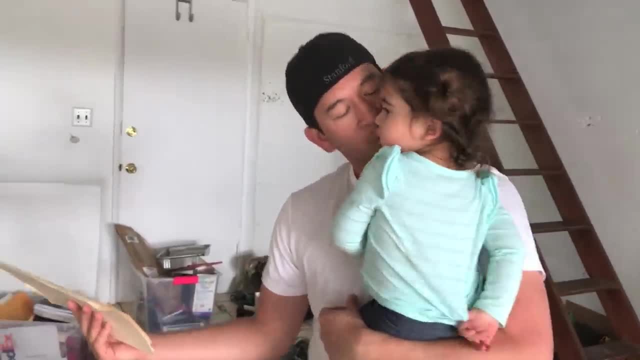 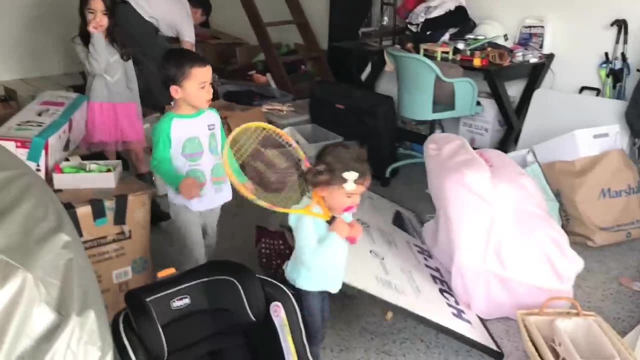 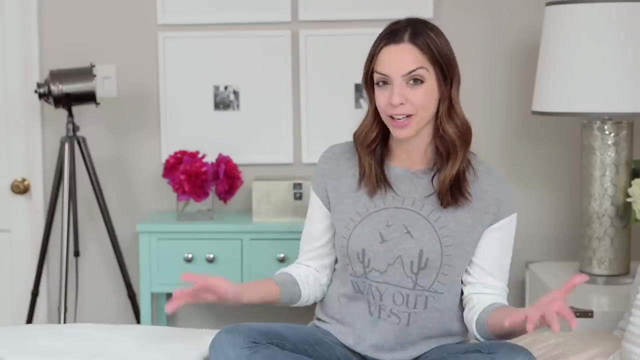 to tackle. Can you help me? No, We gave Ross some moral support. You can do it, dad. A beverage of his choice, And then I took all three kids out with me. While we were there, we got some bins and we were very proud of the progress when we returned. Good job, So finally we 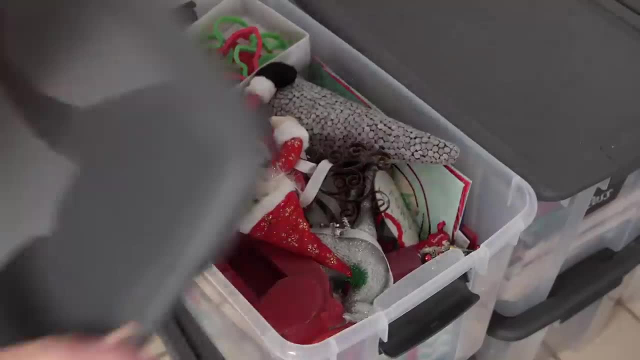 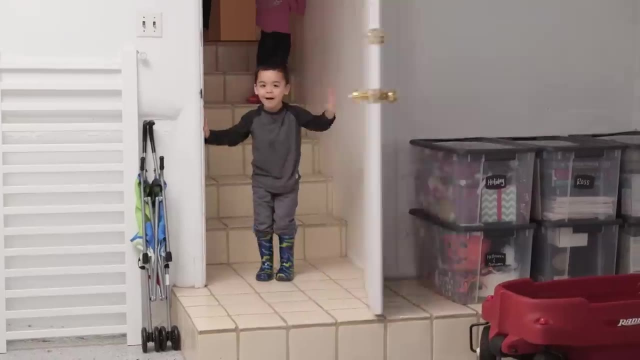 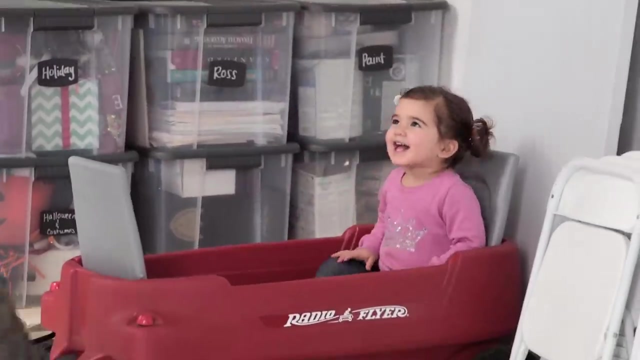 took all the things we were keeping and put them in these bins, like costumes, holiday decor, sentimental items, and we were able to admire our cleaned out garage, One that you can actually walk through and maybe even park two cars. Yeah, Crazy to think about how it started before. 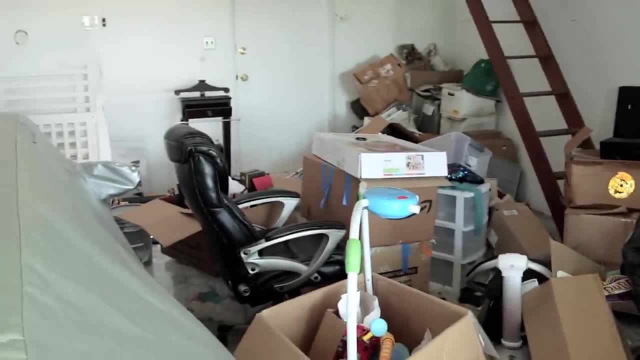 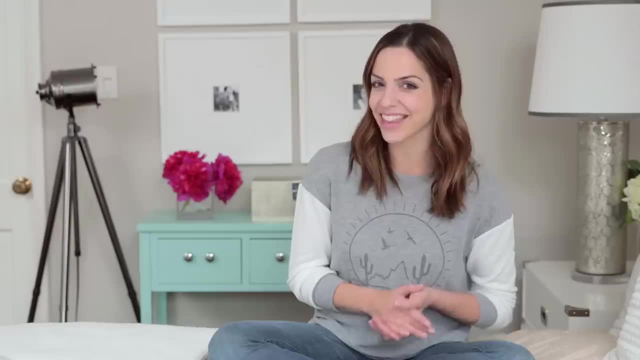 Yes, let's take one more. look Feels so much better now. So if you guys are in the same position, I hope this inspires you and gives you some tips on how to tackle your garage. Thank you so much for watching. We'll see you next week. Bye.